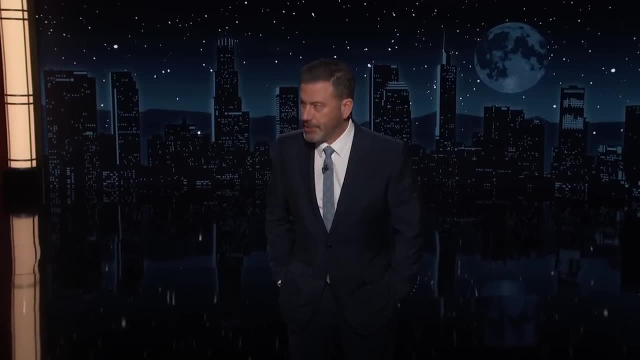 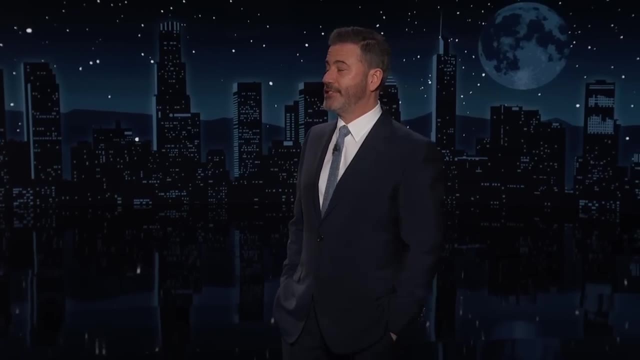 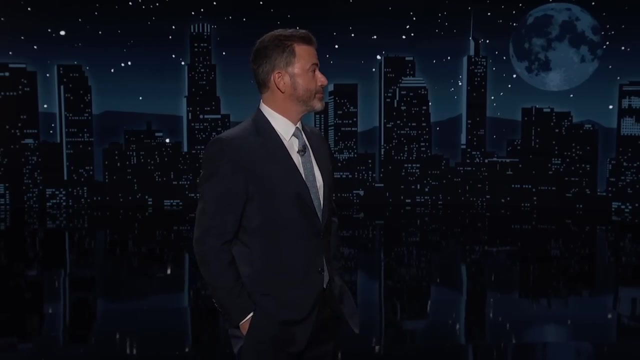 Thank you for watching. Thank you for coming Welcome to Hollywood. You know what I have to say. I really appreciate that. It was a tough day. God, I miss OJ so much already. I really do. As most of you probably know, the big story was that OJ Simpson went to hell today. He arrived at 6.04 this morning- Turns out not much different than Florida. It's rare that a celebrity as famous as OJ was doesn't get an outpouring of love after news of his death, but it makes sense. 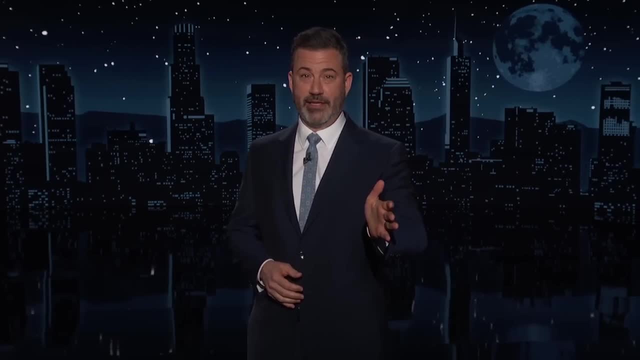 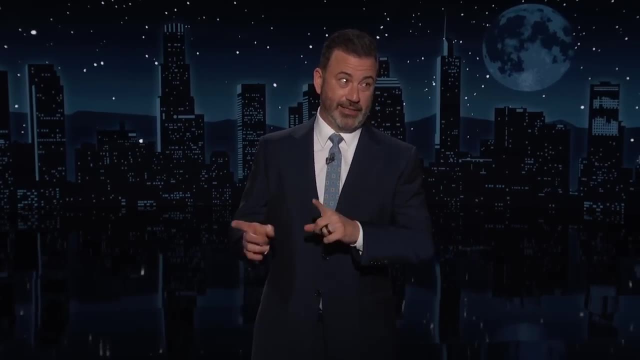 OJ. this is from his old friend, his former very good friend, Caitlyn Jenner tweeted: Good riddance, OJ Simpson. Bruce Jenner loved OJ Caitlyn, not a fan. Very tough week for LA. 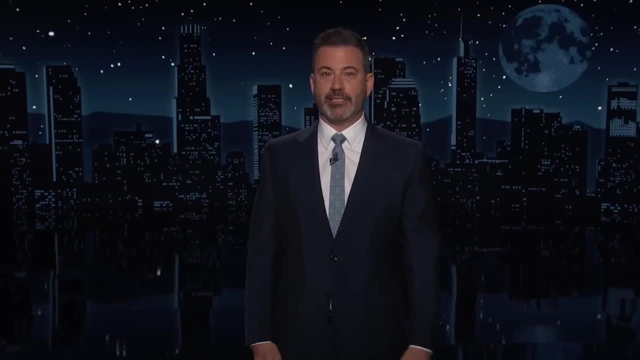 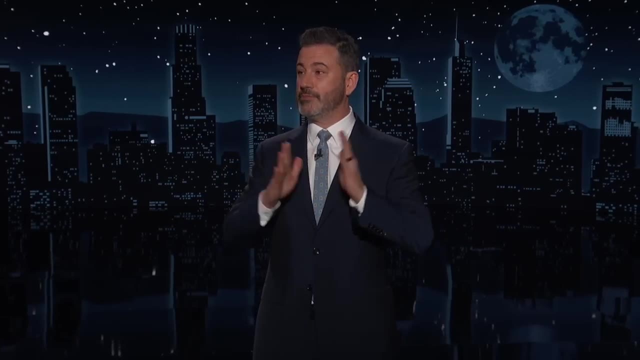 First we lost the 99-cent store and now this It's Hey. we have a special tribute to the juice and all the madness that surrounded him in just a bit. But first we go to Washington, where the mood was celebratory. 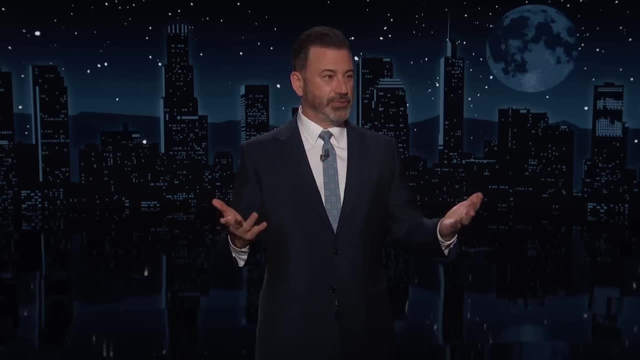 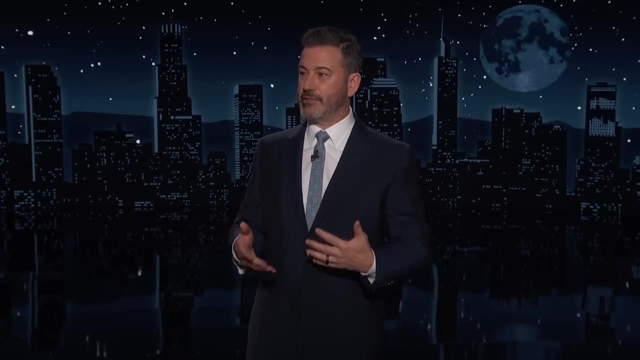 The prime minister of Japan, Fumio Kishida, was in town. They had a state dinner. I don't know. This prime minister- I had no idea- at one time lived in New York. He lived here when he was a child and he reminisced about that time in his life today, before a joint session of Congress. 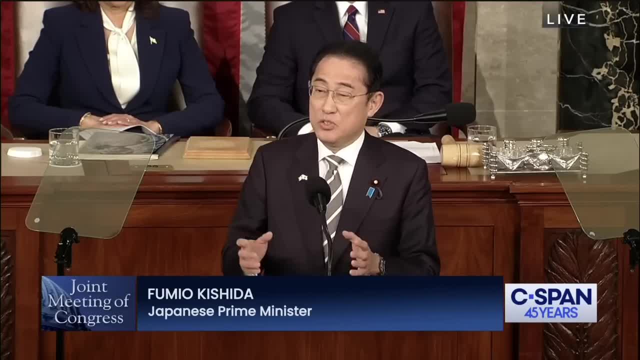 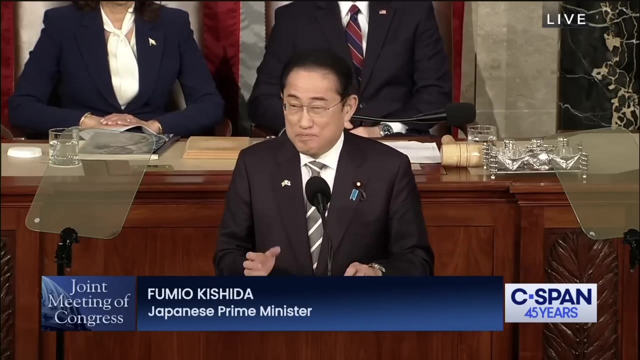 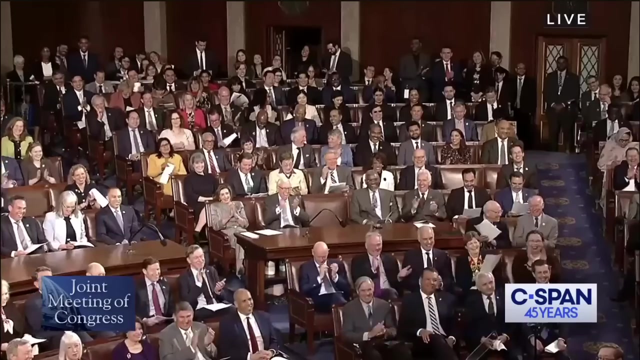 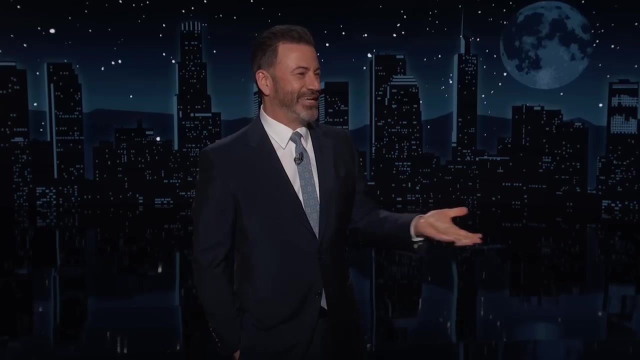 I and I remember things that were strange, Strange and funny to a little Japanese boy, like watching the Flintstones. I still miss that show, Although I could never translate. You know what? What a delightful man Who would have guessed the only leader who could finally bring both sides together would be from Japan. 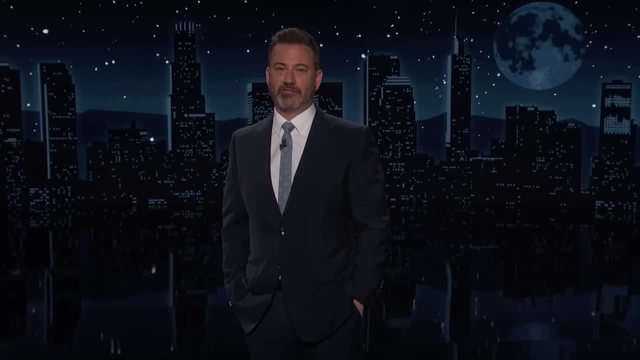 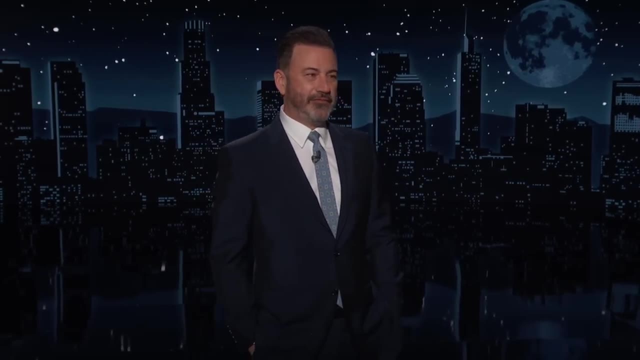 You know things are not looking good for yabba-dabba doofus Donald Trump. His um The porn star hush money trial starts Monday. All his many last-minute efforts to delay it have failed. His only move left is to have sex with everyone in the court and pay them $130,000 to get their mouths shut. 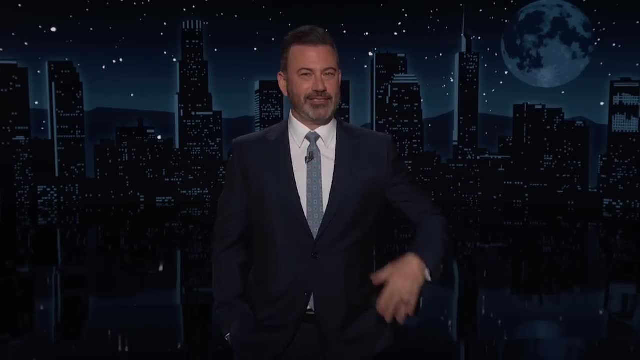 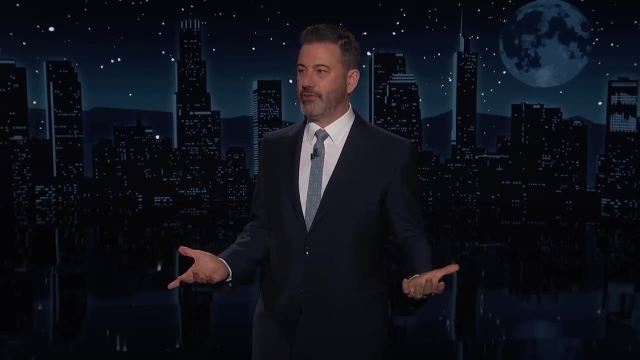 Trump lost three appeals in the last three days. He does this in every trial. to gum up the mechanism. he keeps challenging and challenging and it works. All his trials are behind schedule and most now won't likely happen until after the election, if at all. 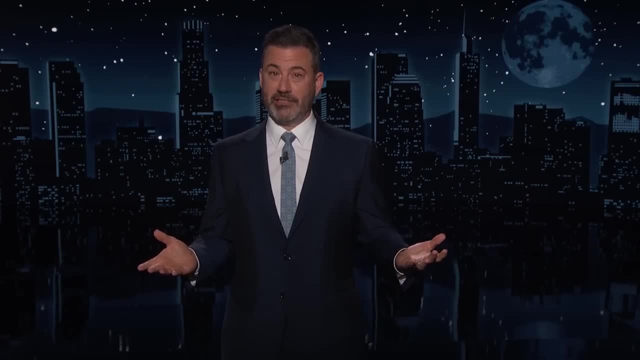 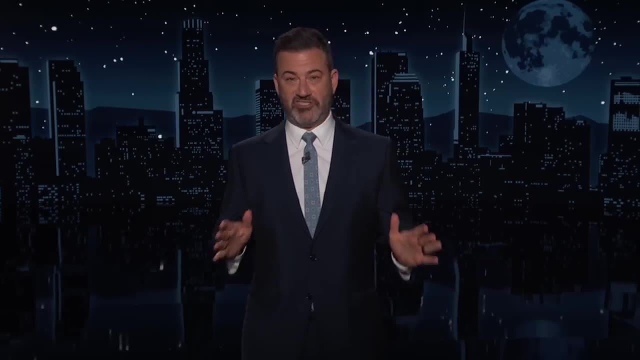 Which I don't know, seems like quite a lot of due process for a witch hunt. to me It's like we can't burn this witch. yet Her attorneys are saying the water we use to see if she floats wasn't distilled. 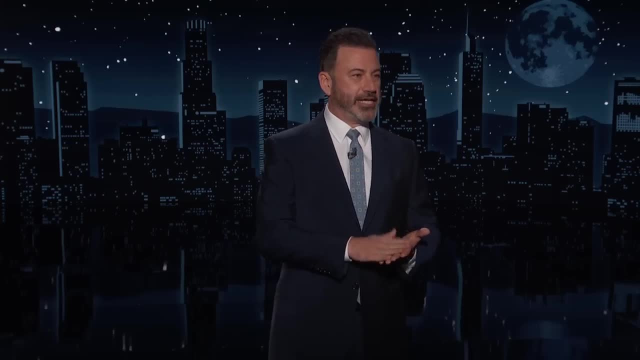 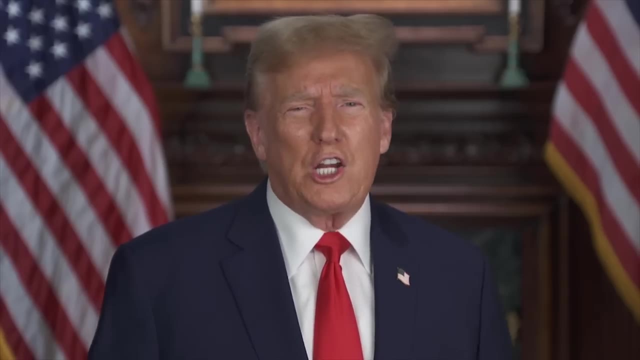 But you know what they say: if at first, second, third, fourth, fifth, sixth, seventh, eighth, ninth or tenth you don't succeed, cry, cry again. At what point are the actions of a sitting president using lawfare and weaponization against his opponent? 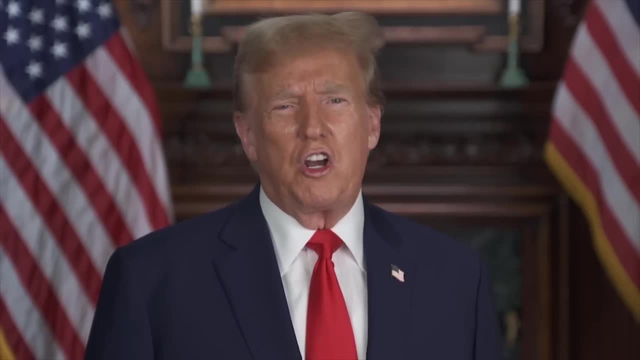 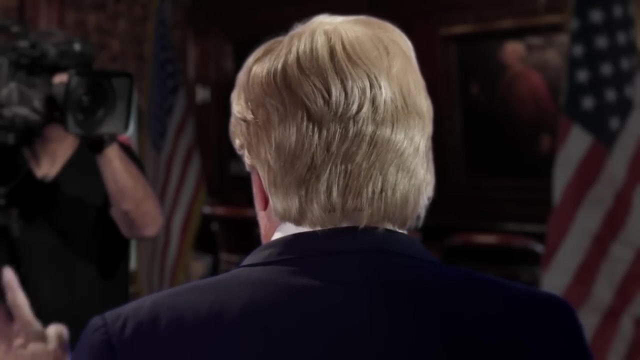 for purposes of election interference considered illegal. I believe, as do various highly respected legal scholars, that Crooked Joe Biden has long since crossed over that very sacred threshold. He is a criminal, He is a horrible president. He can't put two sentences together. He can't do anything. 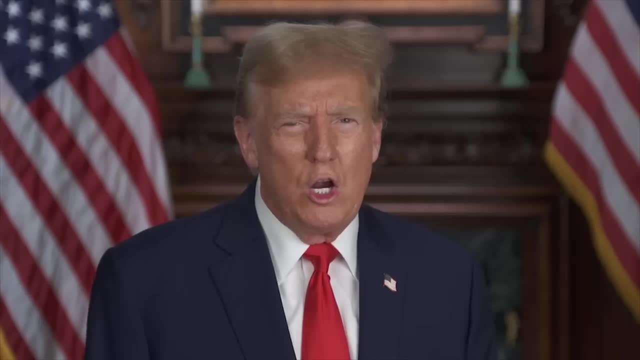 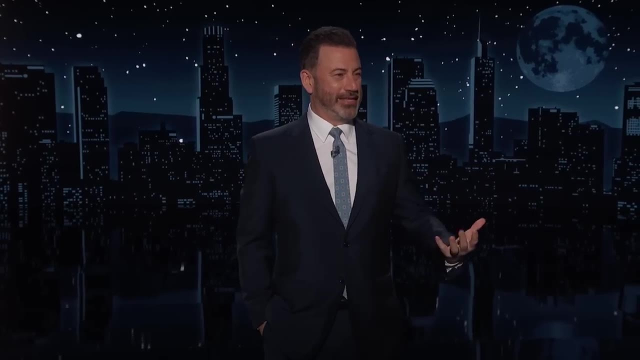 So they weaponize government and they take me to court on bulls**t. Right Biden simultaneously can't do anything. Right Biden simultaneously can't do anything. Right Biden simultaneously can't do anything And is a ruthlessly calculating criminal mastermind. 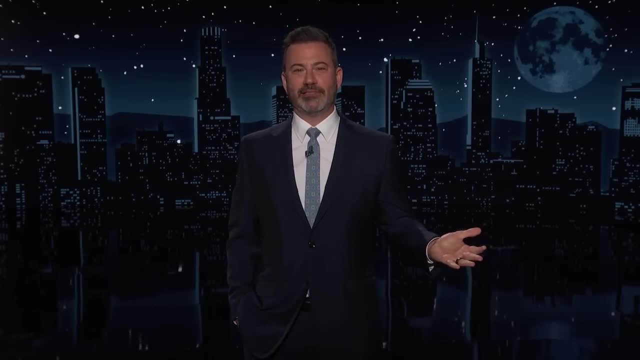 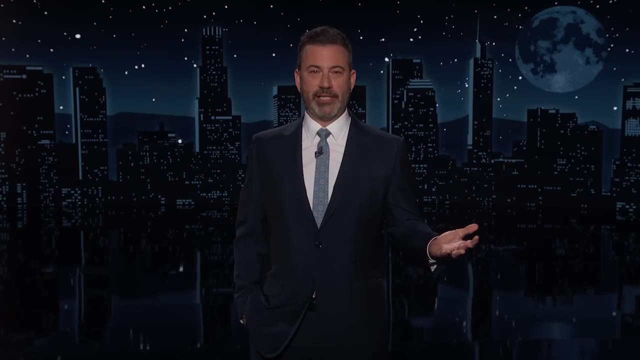 It makes total sense And by the end of the week he'll be saying: Joe Biden's the one who had sex with Stormy Daniels, not him At Mar-a-Lago. tomorrow, Donald Trump and Speaker of the House Mike Johnson will hold a joint press conference on election integrity. 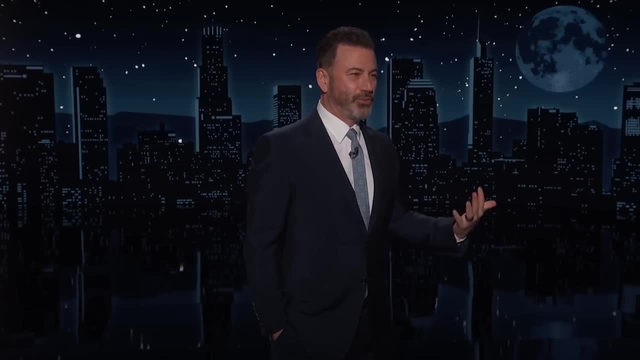 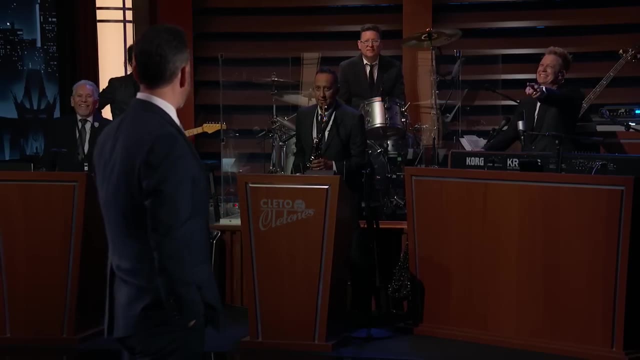 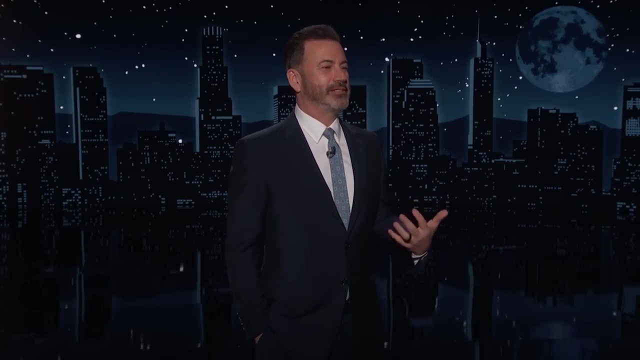 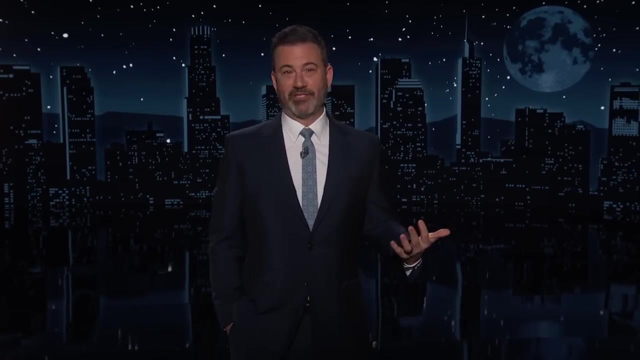 And that's not a joke. Tomorrow, Trump and Mike Johnson really are holding a press conference to talk about election integrity. I just told you it's not a joke. Okay, never mind. Trump has to make his speech about integrity tomorrow because, starting Monday, he'll be in court for cheating on his wife with a porn star shortly after Melania gave birth to their son. 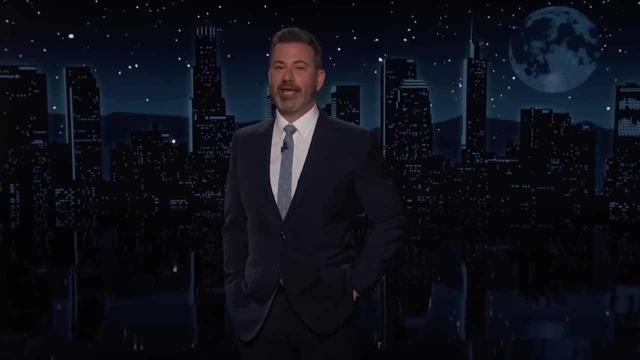 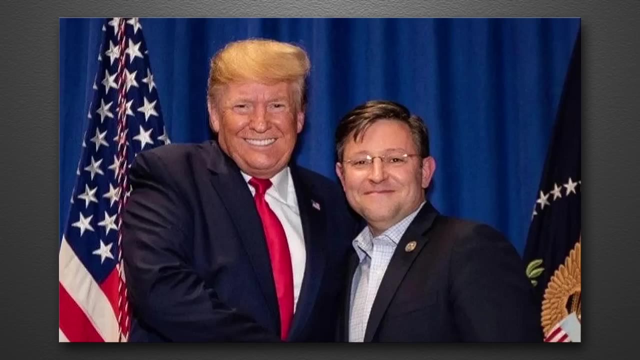 So time was of the essence here. And Trump and Johnson, they are quite a pair. They don't just act like a ventriloquist and his dummy, They look like one too. What's going on? Is Trump tickling his belly? What's going on? 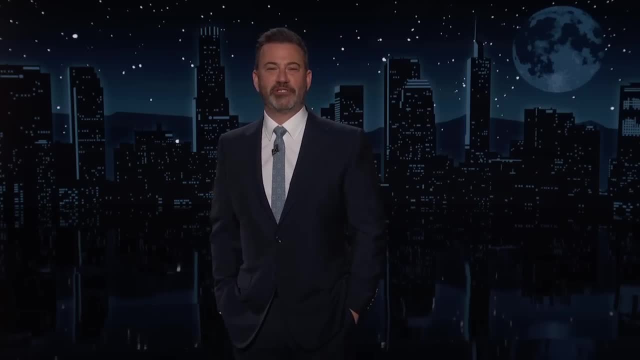 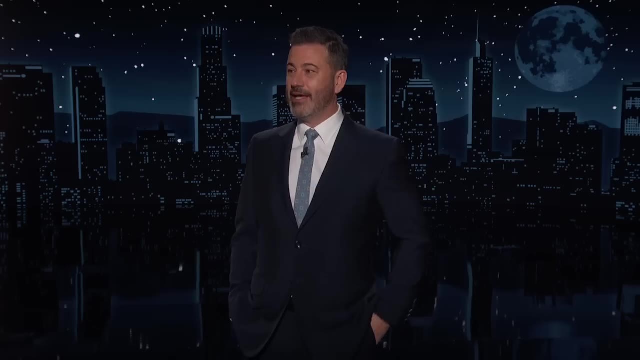 What's happening now? Now, this comes in a moment when Marjorie Taylor Greene, who is Trump's second biggest fan after himself, is actively threatening Mike Johnson And Johnson's hoping if he starts hanging out with Trump more, she'll stop taking his lunch money. 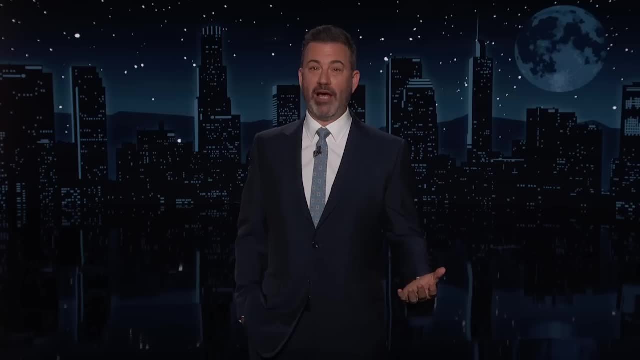 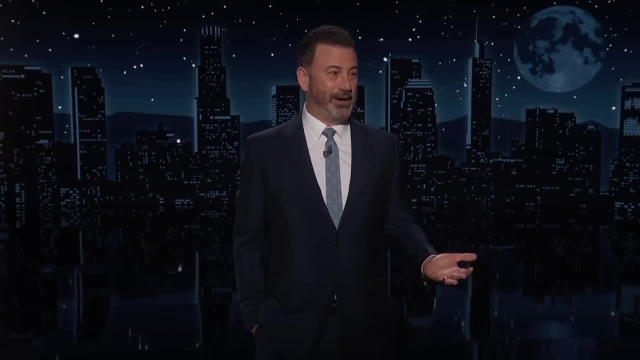 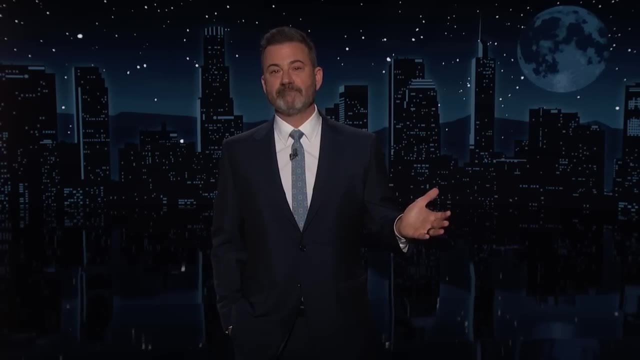 Ron DeSantis, as you know, spent the better part of the year trashing Trump. Now he wants to raise money for him, And there's actually a very good reason why He's a little bitch. He's- um, It's another chicken with his backbone removed. 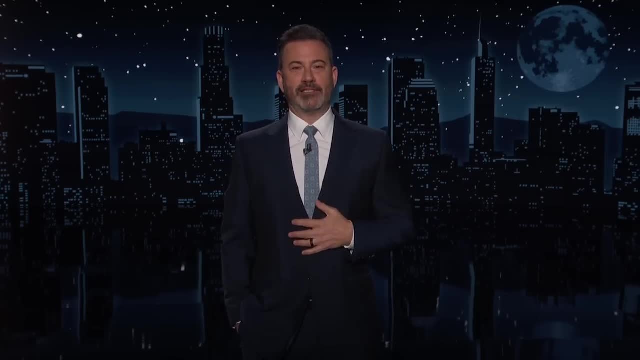 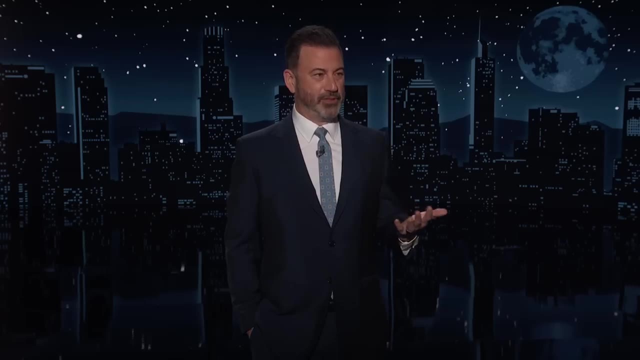 They call it spack-talking. I believe, Speaking of the spineless, Trump's occasional concubine, Ted Cruz, is having a tough week. A watchdog group named the Campaign Legal Center filed a complaint with the Federal Election Commission saying that the company 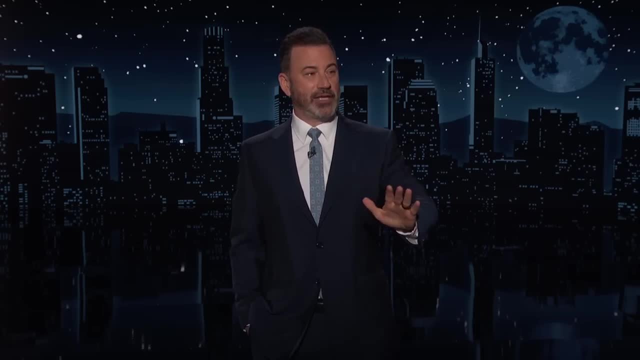 that produces Cruz's podcast has been funneling money to his SuperPAC, which would be a violation of campaign finance law. You can't like sell advertising and give that money to yourself. Ted's SuperPAC is called Truth and Courage, which is rich. 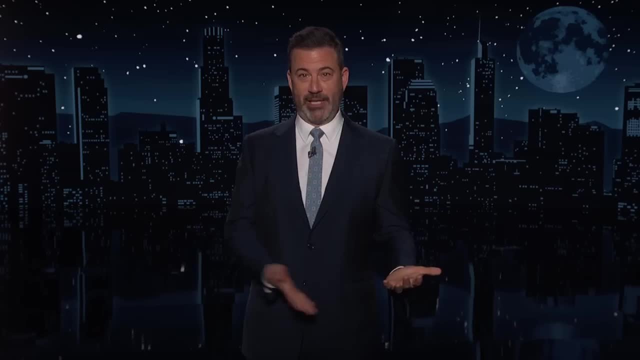 coming from the guy who fled to Cancun during a snowstorm and blamed it on his daughter. His campaign claims no laws have been broken because Ted does the podcast as a volunteer. They say he appears on the show three times a week for free. 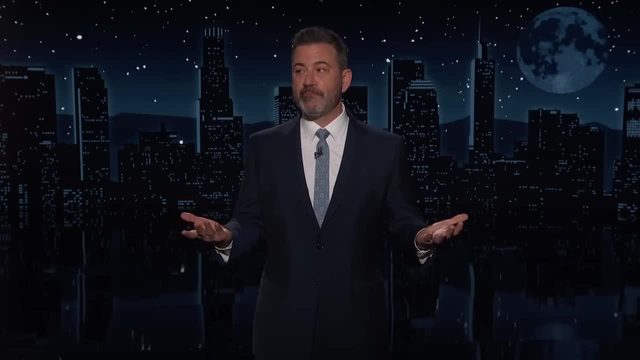 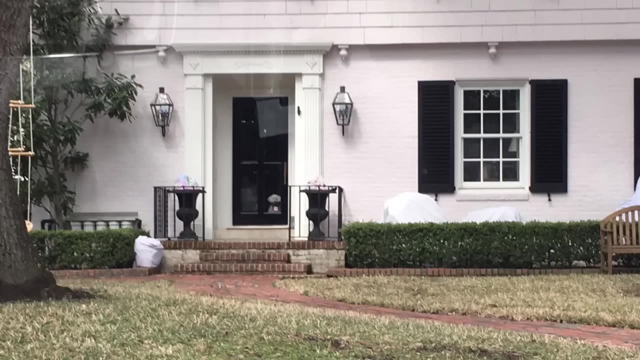 The same way his face appears in our nightmares. But that's a very loopy loophole, And the watchdog group that filed the complaint- this is interesting- is led by the same watchdog, Ted, abandoned in the storm. Snowflakes Bite him snowflake. 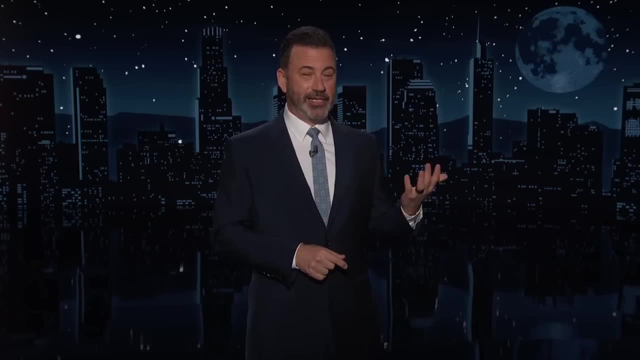 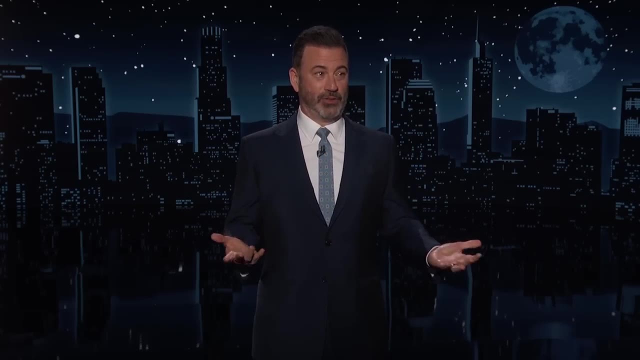 In Arizona, I'm sure you heard- the state Supreme Court decided it was okay to enforce a law from 1864 that bans abortion. Yesterday Republican lawmakers in Arizona refused to repeal that law, And if you're wondering what kind of people would do something like this, 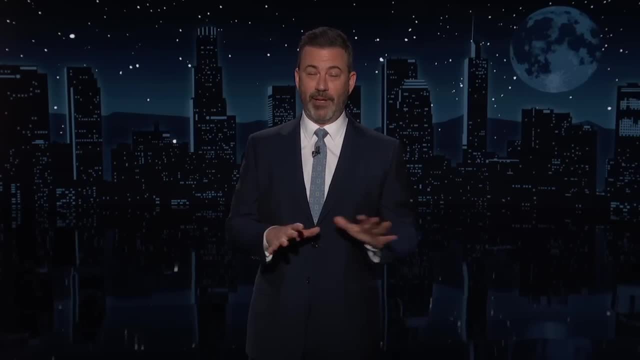 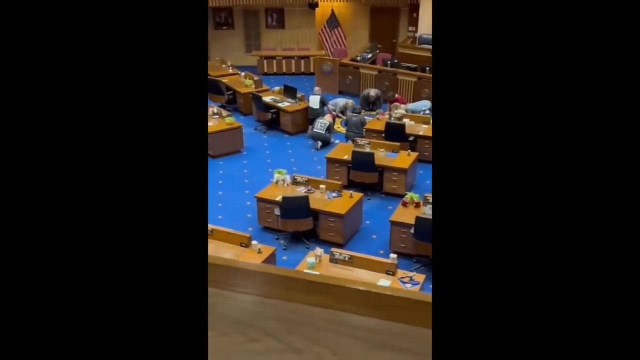 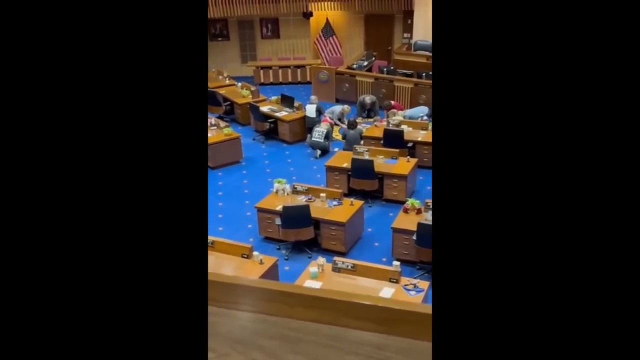 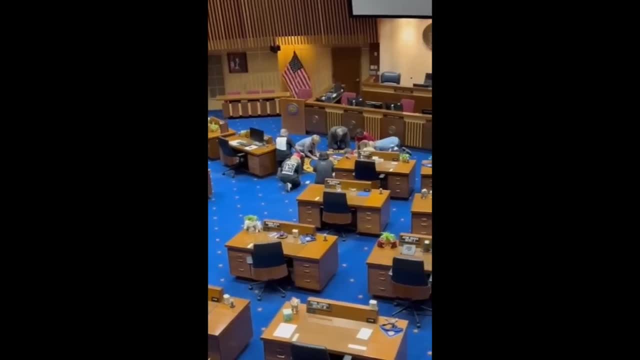 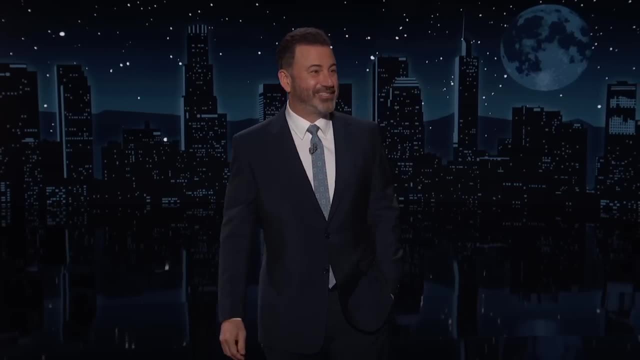 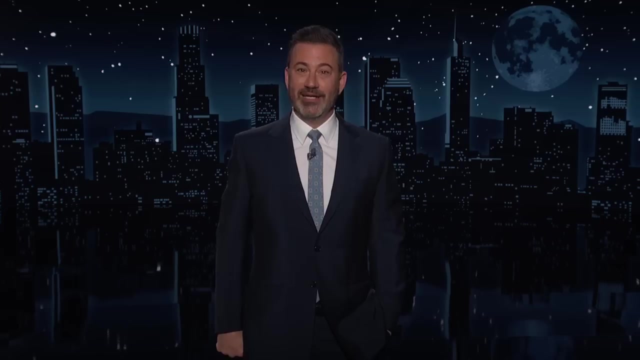 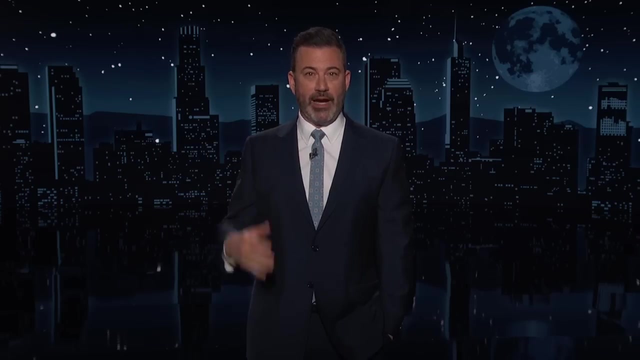 And guess what It worked. These are the people taking over your womb right there drooling on the carpet in Arizona. President Biden condemned the decision. He said he wasn't in favor of this law when they passed it back in 1864, and 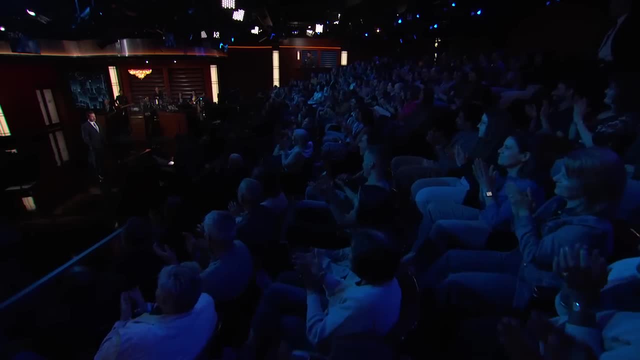 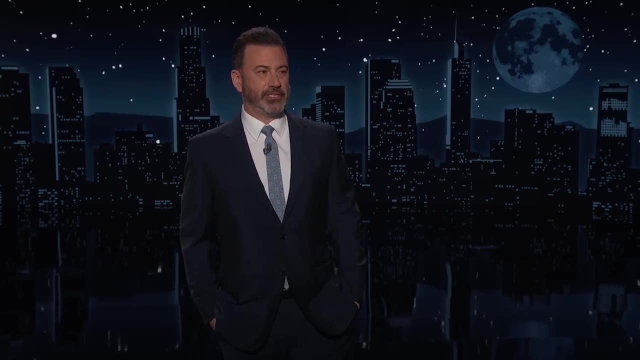 he's not a fan of it now. But the Biden campaign: they're on a very different page. Yesterday they launched a new program to engage voters in the LGBTQ plus community. It's called Out for Biden Harris, which is a clunky title. 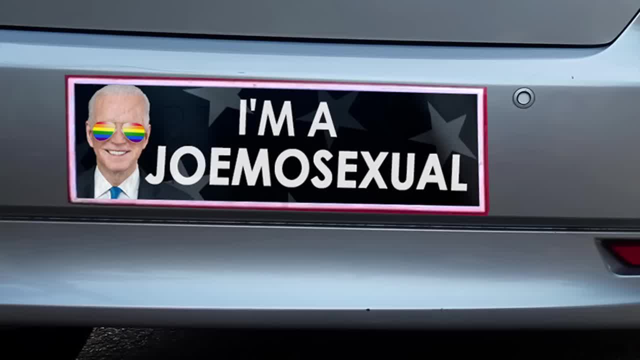 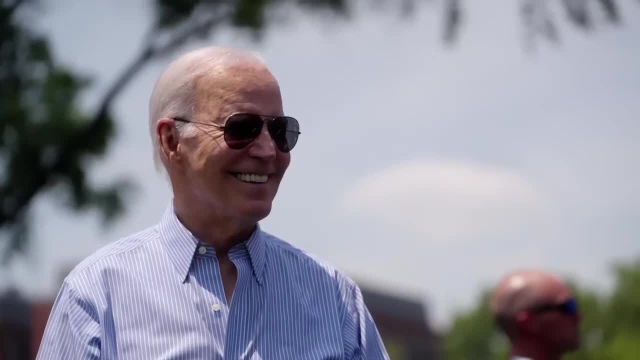 but definitely better than their original slogan, which was: I'm a Jomosexualist, But Team Biden sees an opportunity here and they're going all in. What's up, bitches? It's me, Joe Biden, And I'm excited to announce the launch of Out for Biden. 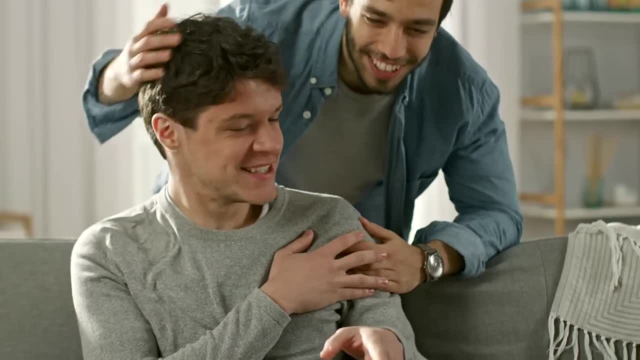 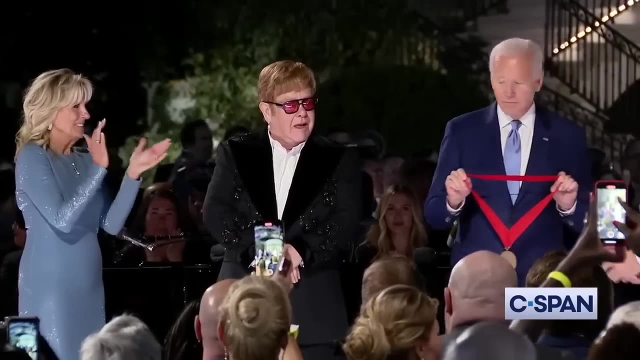 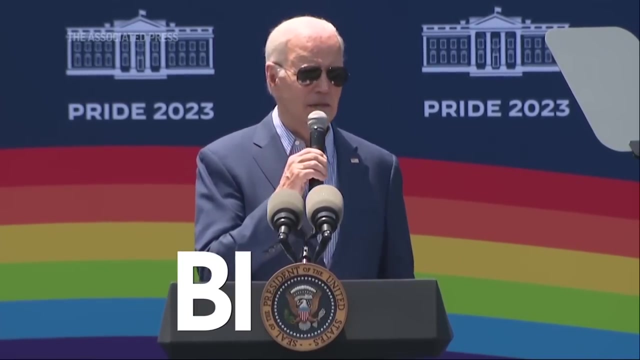 It's a new campaign all about you LGBTQies out there. Listen, I may be straighter than a bamboo fishing rod, but I'm the most gay-friendly president in history. My dear mother always used to say: you can't spell Biden without bi, and that's the T. 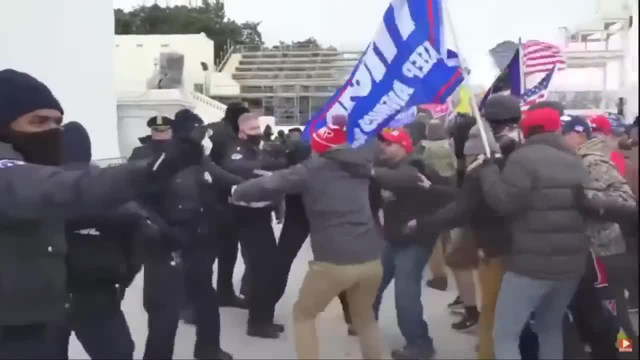 If Trump wins this November, democracy as we know it will sashay away. That's why I'm asking you to vote for me. Remember when I accidentally forced Obama's election to be a Republican? This is why I'm asking you to vote for me. 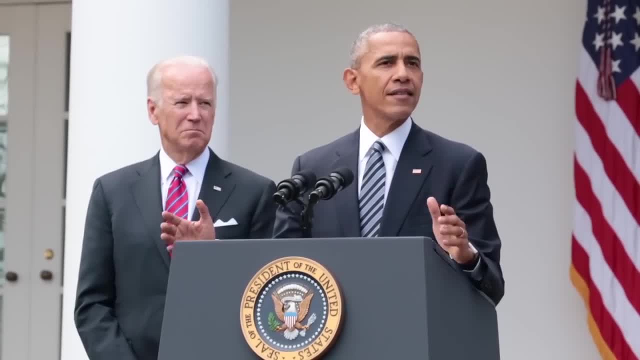 Remember when I accidentally forced Obama's election to be a Democrat? This is why I'm asking you to vote for me. This is why I'm asking you to vote for me. Obama to support you people. before he was ready, BO was POed. I got my bottom reamed. 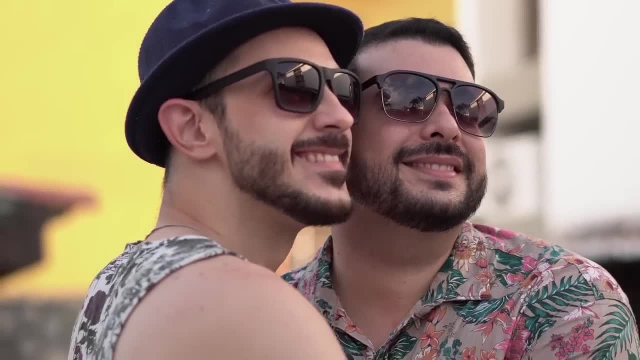 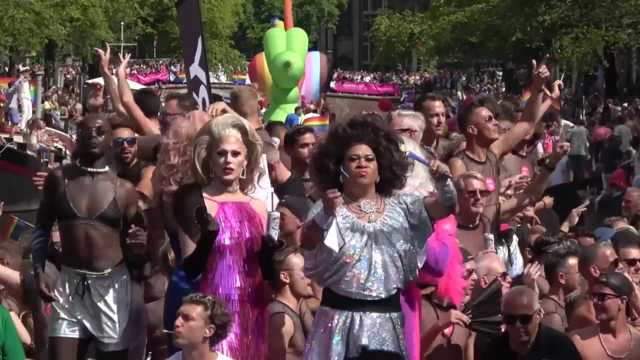 and not in a good way. So, whether you're a teddy bear, a twinkle little star or an indigo girl, no matter if you're a she-her, a they-them, a zaddy or a parade gay, I love you And. 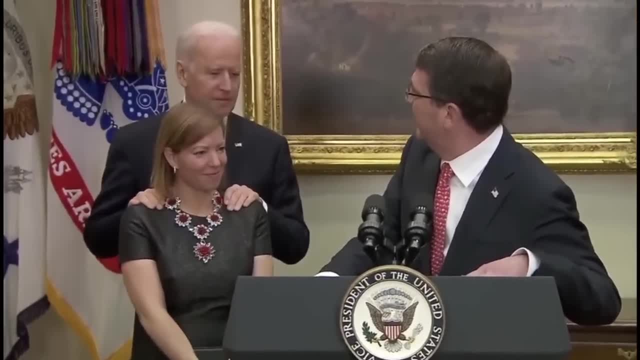 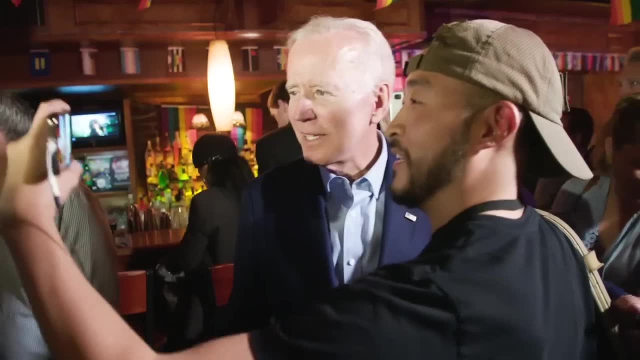 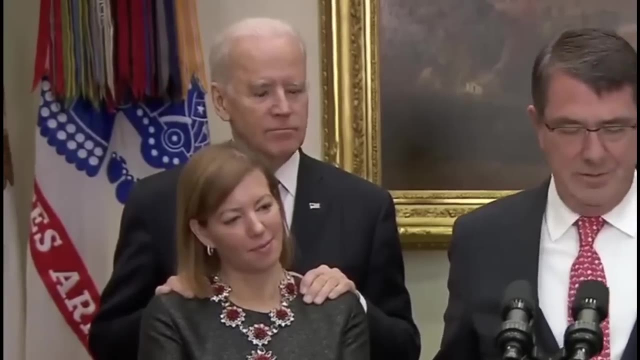 I want to sneak up behind you and give you a shoulder rub, no matter who you are or if you want it. So please vote yas, queen. for me, Joe Biden, I'll make sure the White House stays the down boots hunty. I may be sis, but I've got your back. sis, I'm Joe Biden. 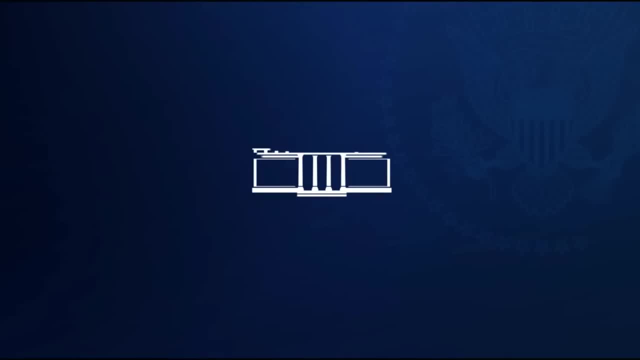 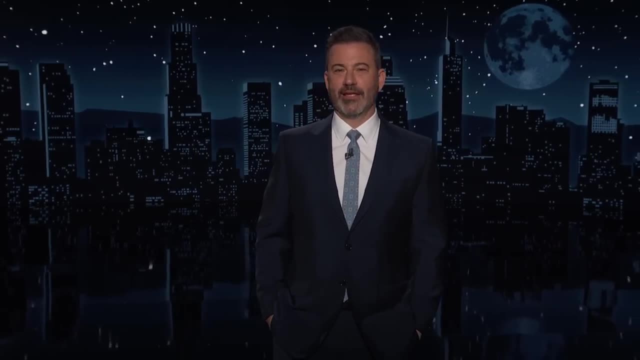 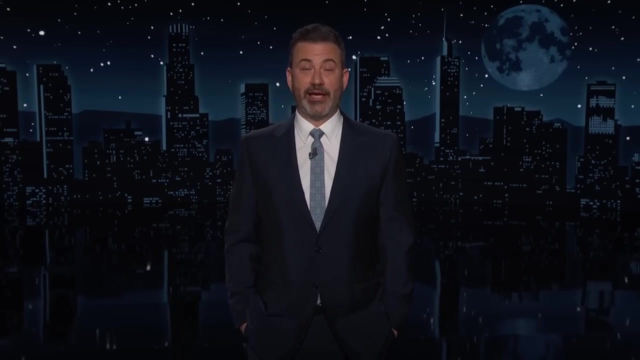 and I ate that up and left no crumbs. What the hell did? I just say I don't know either. I think You said it. well, All right, back to OJ. OJ, OJ, OJ. Before there was Donald Trump, before there was DJ, we had OJ. It's hard to explain. 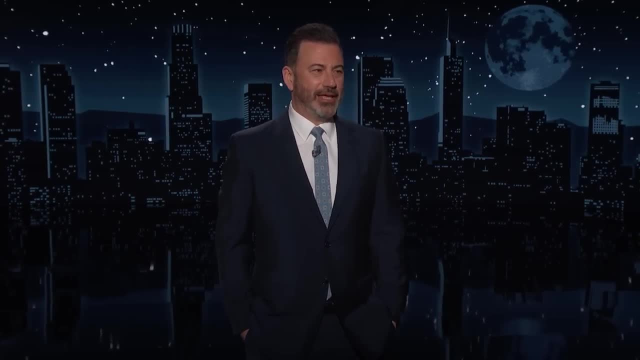 to people of a certain age how big this OJ story was. It was everything. It changed the way news was covered. There was a constant OJ nonstop on every channel, and we made the most of that with our old pal Jake Bird, who was very supportive of OJ and Michael. 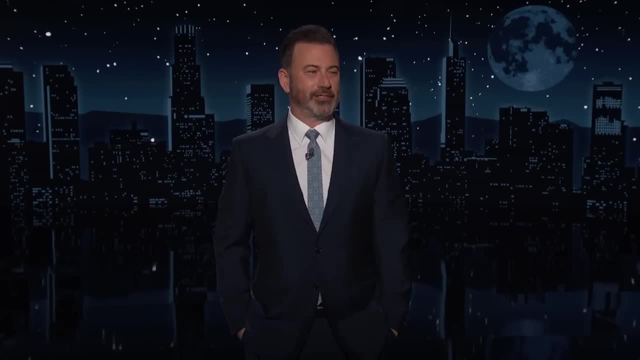 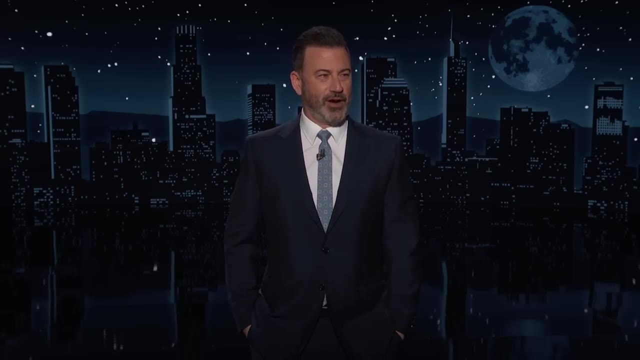 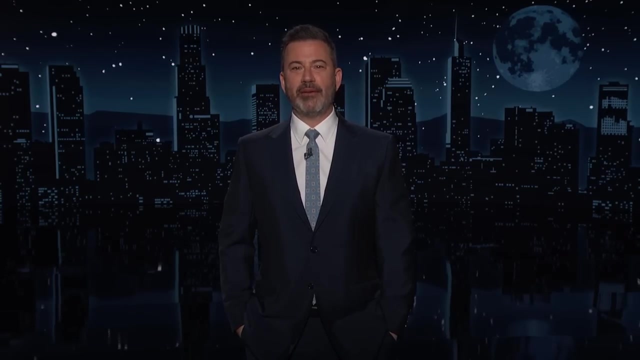 Jackson in Paris. So any time a celebrity got arrested, Jake was there to protest, And it happened in New York For the first time. OJ committed a national crime and the Police Department of Virginia has yet to stand up for someone like Jake Bird. 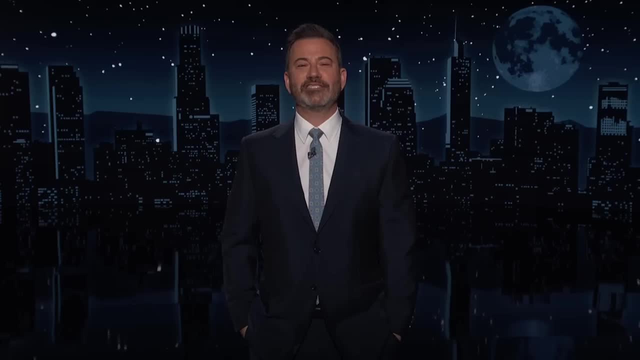 Last year a couple of threats were made to Mr Reynman in Nevada. OJ committed a number of crimes, trying to steal back his own memorabilia in Las Vegas. so we sent Jake Bird, who not only did he cover the story, he became a part of the story. Let's set the clock back now to 2007,. enjoy Jake Bird at the OJ trial. 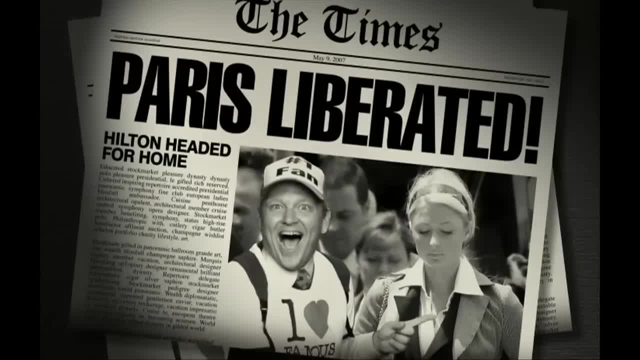 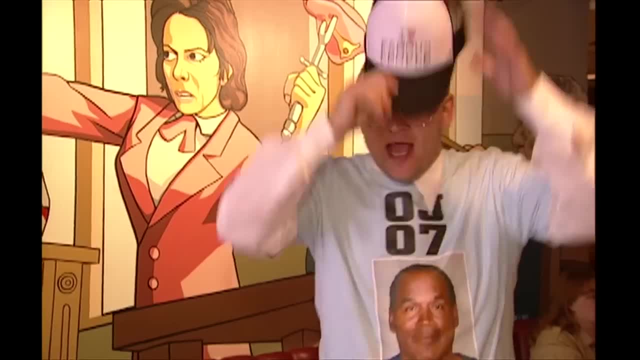 Jake Bird here live in Las Vegas. They called the OJ Simpson trial the trial of the century. Now it's a pain in the neck to see what happens. Stop it, you animal. Should I be in prison because you damned me for doing that? 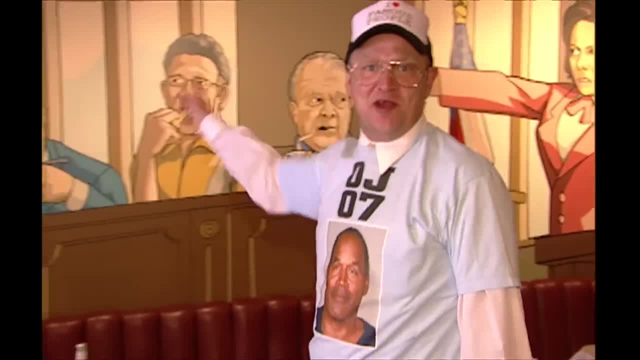 trial, the trial of the century. Now it's a painting on a diner across from the new OJ Simpson trial And look, there's dead Johnny Cochran with his hand on a chicken. Let's go to court, Come on. 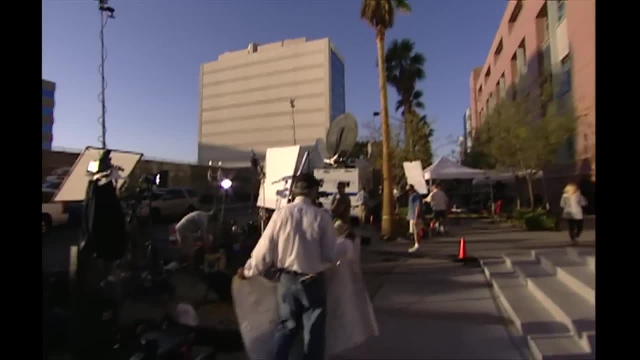 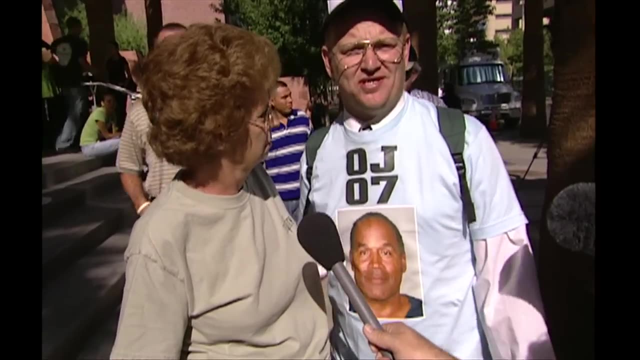 Come on, You're going to catch me. I've been following this the whole time. We're here to support OJ. We know OJ is innocent. He's being railroaded by a biased legal system that keeps African-Americans like us down. 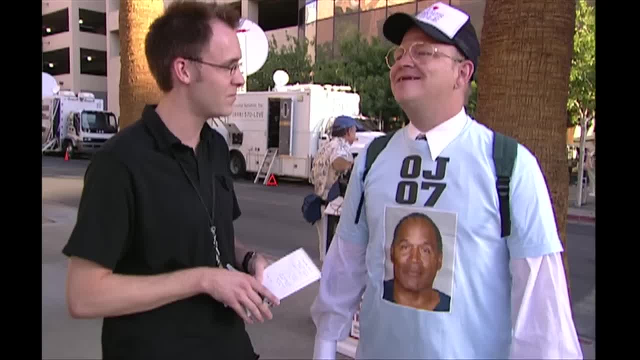 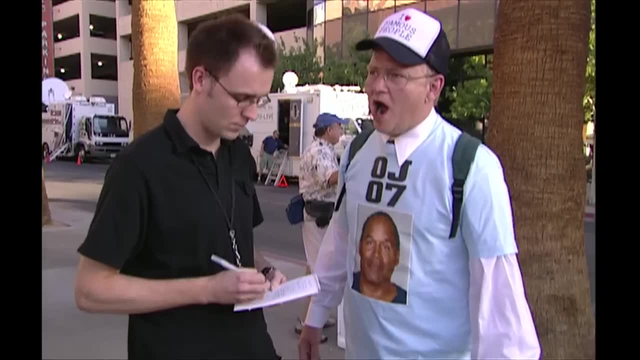 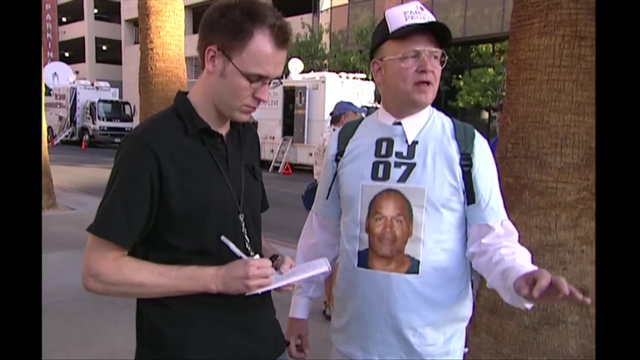 Thank you What. It doesn't matter if OJ broke into a room and committed armed robbery or kidnapping with a deadly weapon. The point is he should be able to get away with this, because he's gotten away with stuff that's way worse. 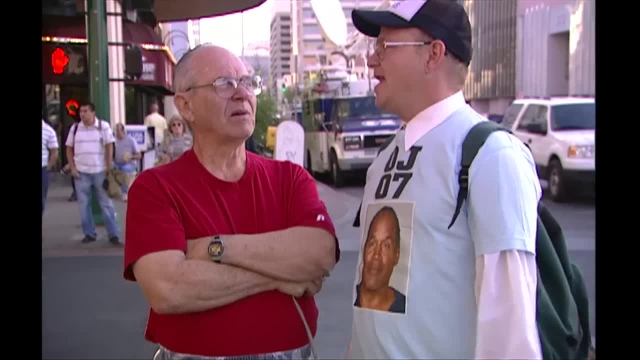 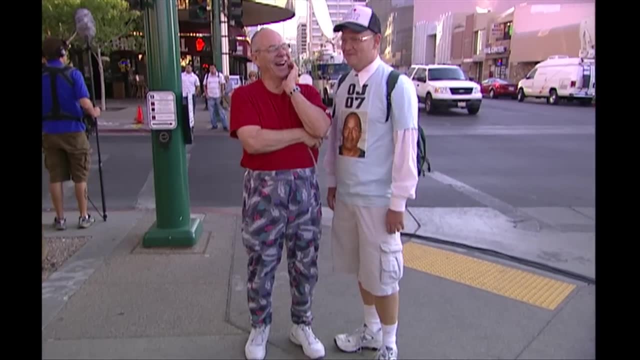 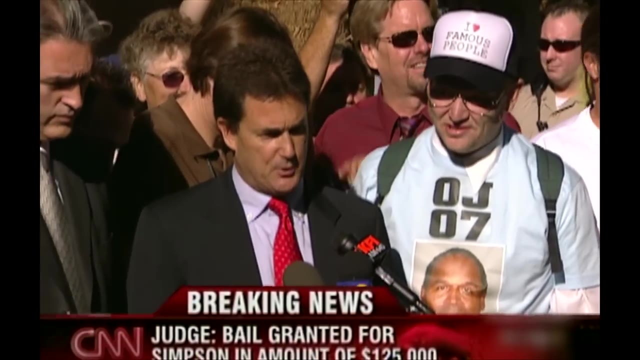 Well, I mean, but Way worse. People get on OJ's case and what You've never made any mistakes I mean. look at those pants Where you from. We expect Mr Simpson to be processed and released. 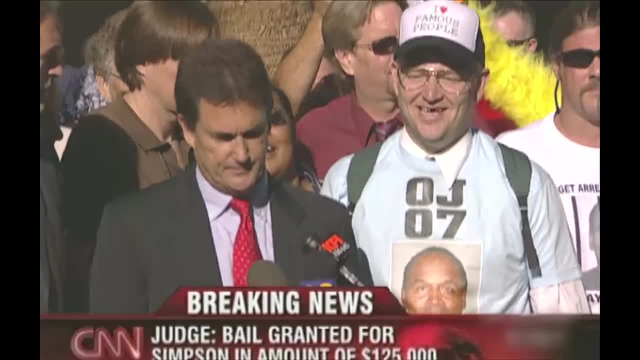 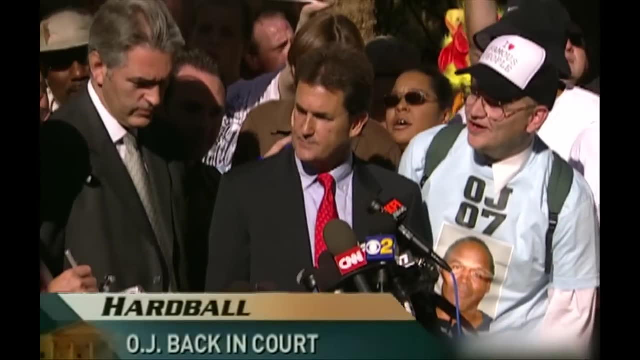 Yes, Fairly quickly, Because you all knew who his lawyer was, This guy right here. Yeah, Is your client innocent or not guilty? I'm not sure there's a difference. in the eyes of the law, He's both dude. 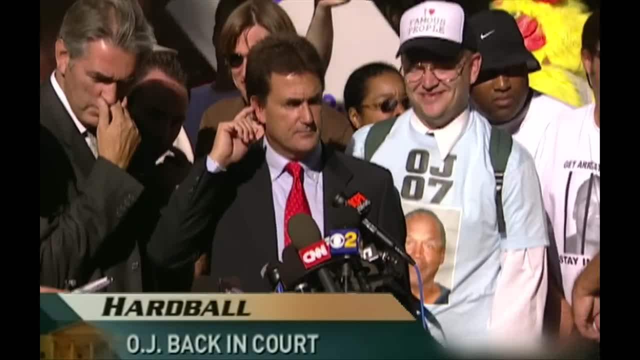 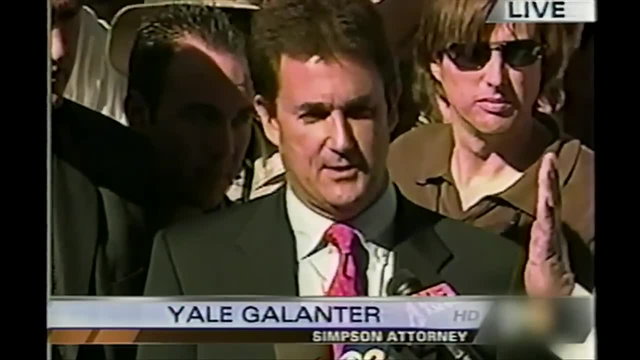 He's innocent and not guilty. Thank you, My only focus up till this point in time has been securing Mr Simpson's release from custody. Nice work, dude Up high. Thank you very much. Yes, right here, Come on, let me hug you. 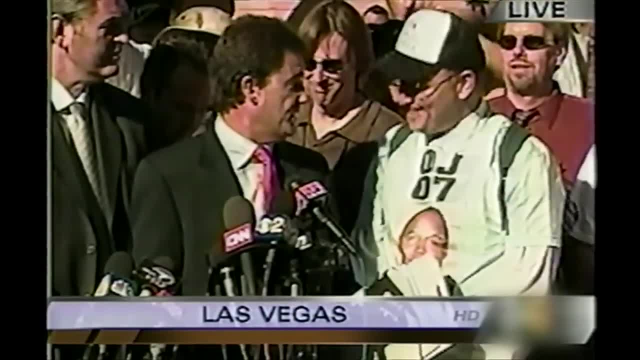 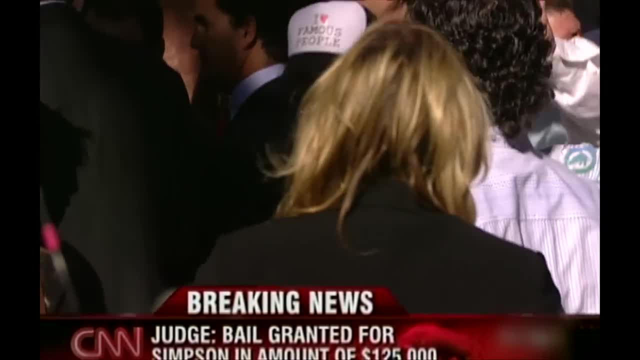 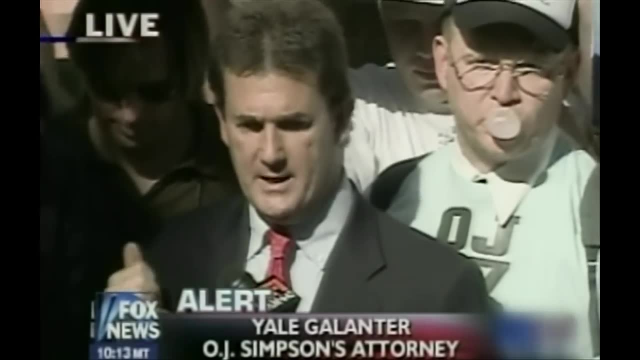 No more questions. Thank you, Mr Pesci. Pardon the sideshow there: Yale Galanter. Yale Galanter, OJ Simpson's attorney, being welcomed into the world of OJ Simpson and the criminal law by a man. 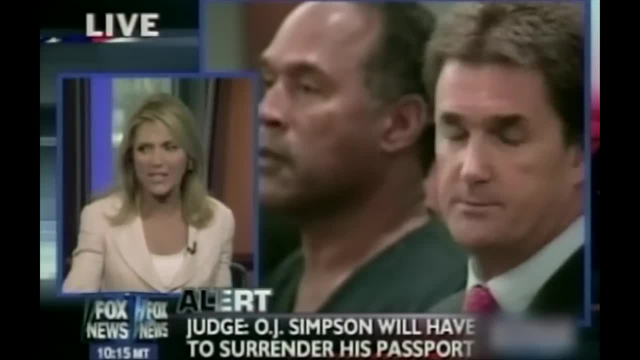 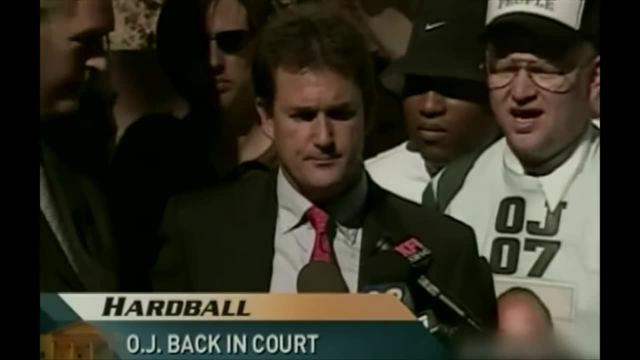 He's wearing an I Love Famous People hat. You saw this cast of characters there: Baseball cap, I Love Famous People. Note the man with the OJ and O.7 t-shirt. He made himself part of the Simpson defense team. 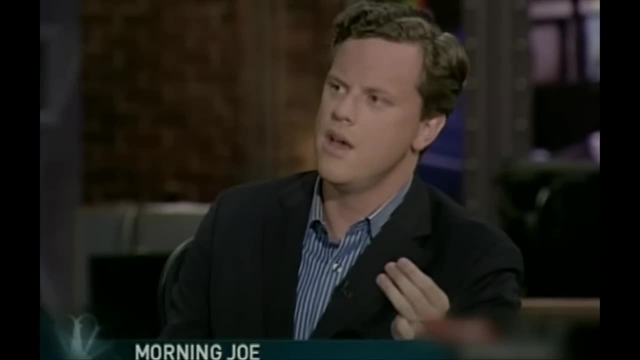 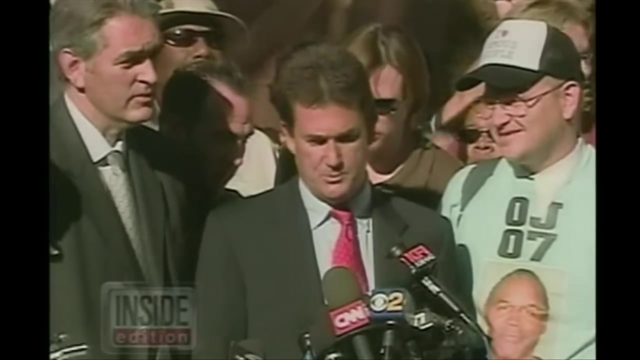 Our favorite part, I think we can agree, of the OJ circus yesterday. It's getting me through it- Mika's man, Jake Byrne. He was repeatedly interrupted by Jake Byrne wearing an OJ t-shirt- Our number one story on the countdown. 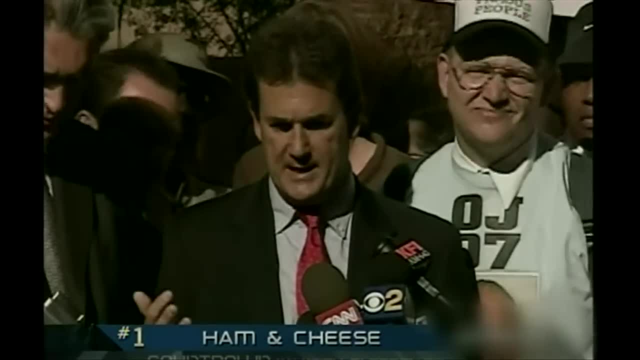 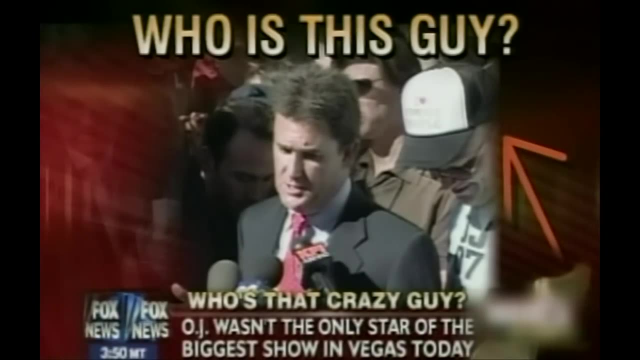 he's the guy on the right, the one wearing the OJ O.7 t-shirt With the hat that reads I Heart Famous People. It was hard to take your eyes off one of the people in the crowd. Fox's Laurie Due has more. 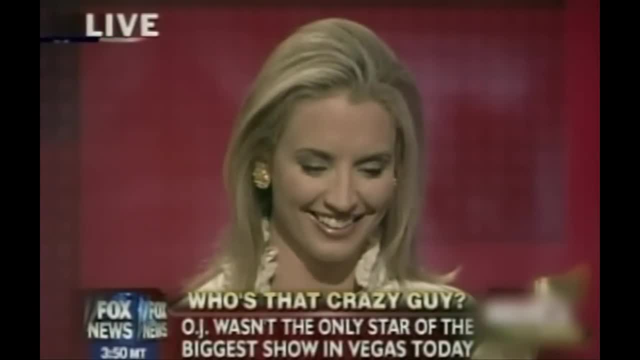 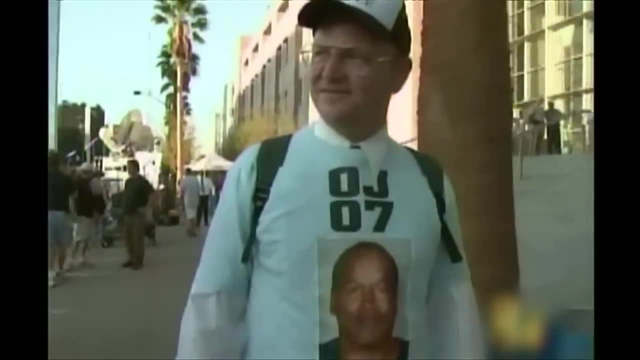 And the man has been getting way more than his 15 minutes of fame. Yeah, John, much of America has been watching these 15 minutes, And I, for one, hope that these 15 minutes are up. So-called celebrity Avenger even showed up. 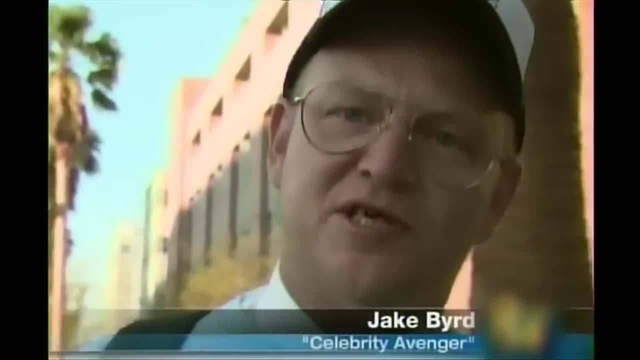 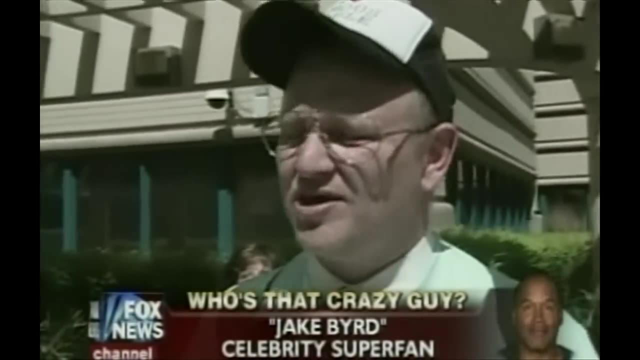 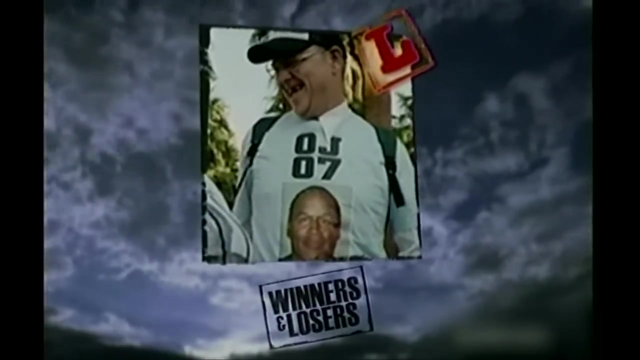 Jake Byrne. I support the famous because they don't have a voice to speak out for themselves. I came out here to let OJ know that all of America, all of America, supports him 1,000%. The big loser of the day, the ultimate fool, Jake Byrne. 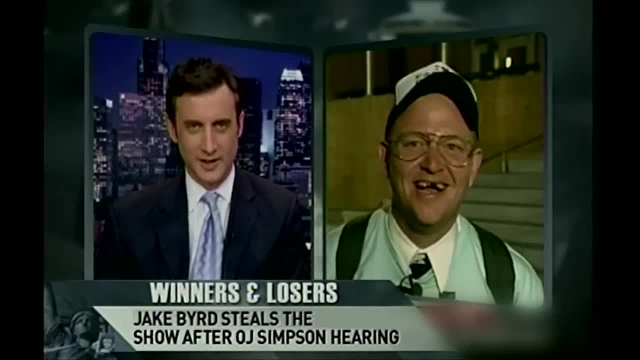 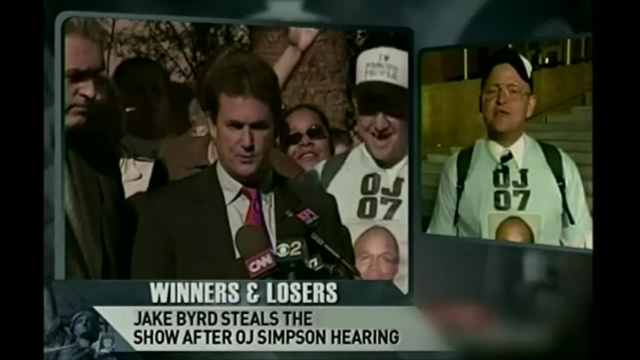 I missed a thing. Am I the winner or the loser? You were the big loser, But you're a winner. I could. I'm a little concerned that you think this whole thing is a joke. Dan Abrams, If this was an OJ joke I'd say: 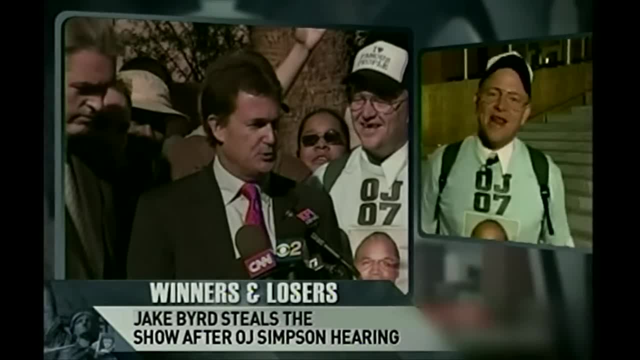 what's OJ's favorite soda Slice. But it's not a joke, OK, Not a jerk. We appreciate you taking the time. Thank you for taking the time to come on the program today. Can I just tell you something? 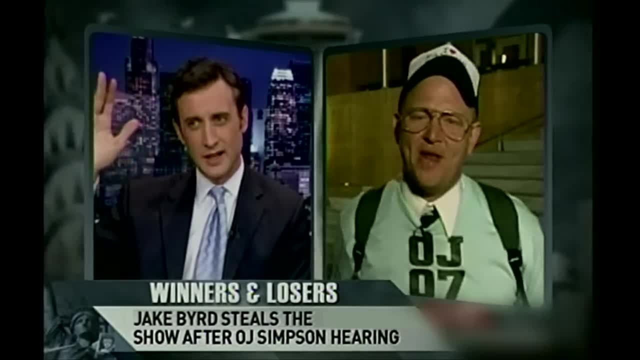 Can I tell you something? I got to wrap it, Jake. This is an opportunity for white people to jump on the knockout to Dan Abrams. All right, I got to go See you. Come on, white people. We've got video now of OJ walking out. 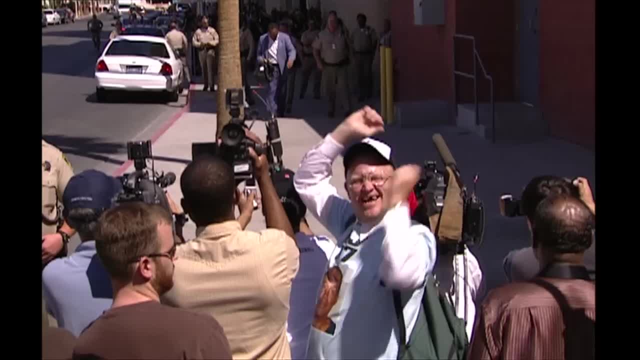 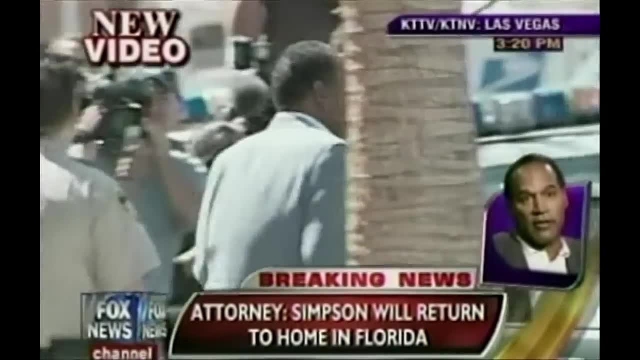 Here it is OJ, back in his suit walking out. There he is Touchdown Simpson. The juice is free. The juice is free, Two for two, See OJ. And he drives American, He drives American. 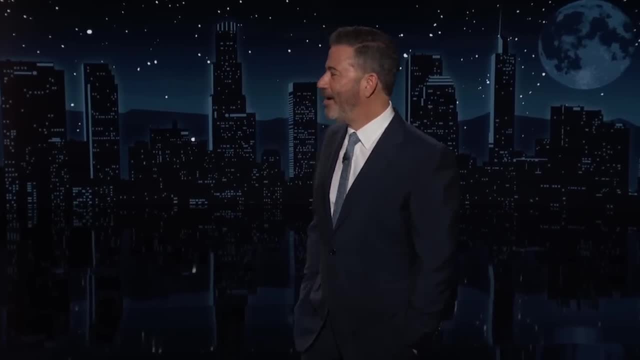 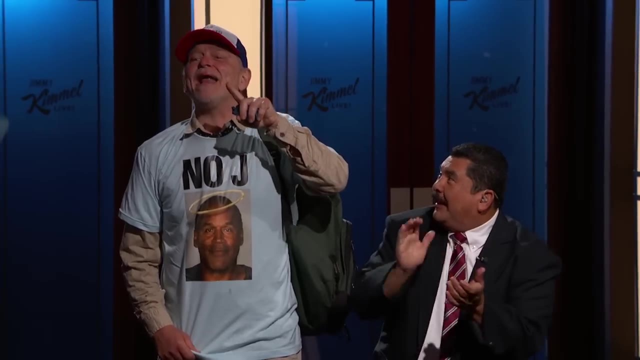 Oh, wow, Oh, my gosh OJ. You know what? I'll tell you something: He might not have been the greatest husband in the world, but he was my buddy. I'm so sorry, Jake, But thank you for being here. 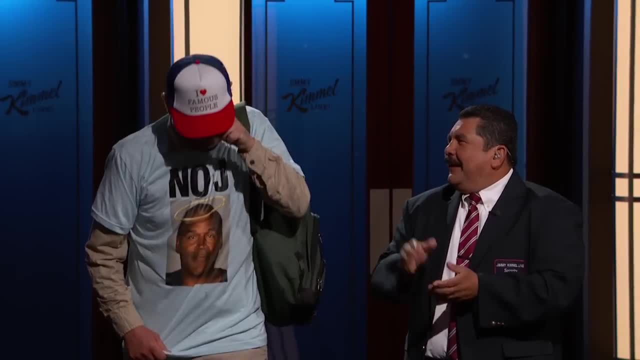 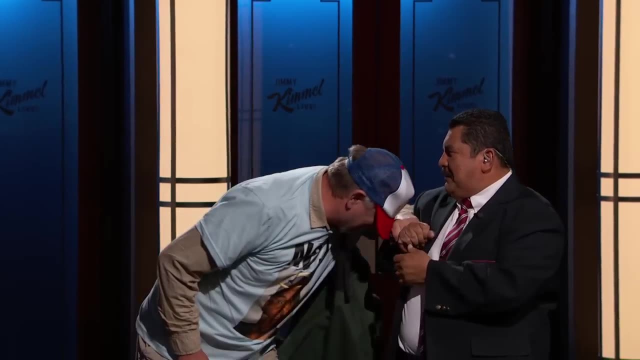 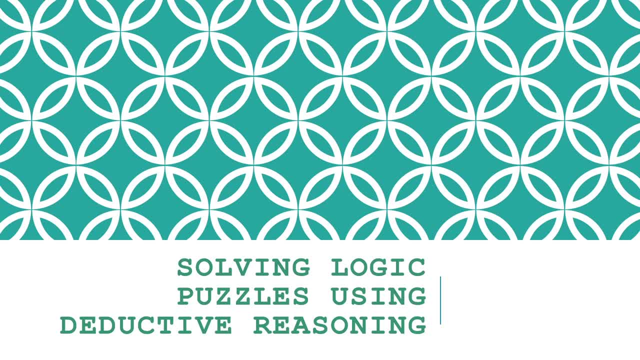 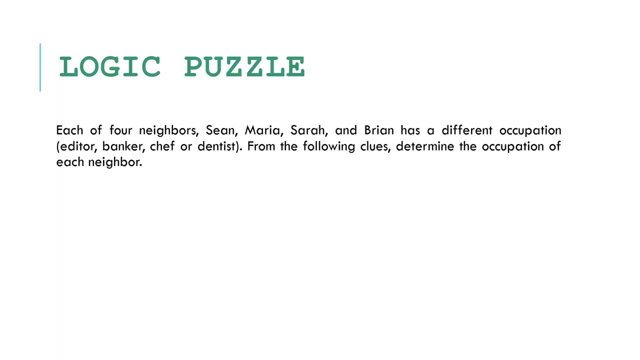 One fun way where we could apply deductive reasoning is when we try to solve logic puzzles. Now, what are logic puzzles? Basically, they are puzzles that we need to use our power of deductive reasoning to solve. So this is an example of a logic puzzle that we will try to solve using our deductive reasoning.